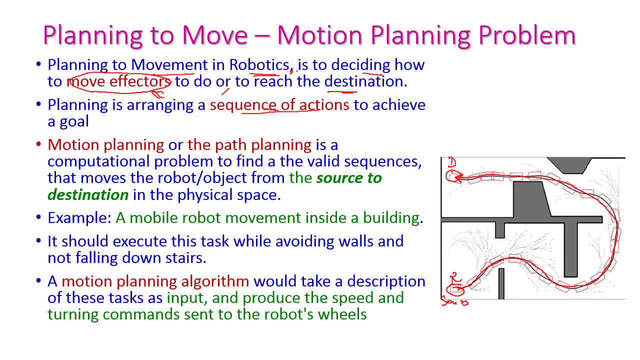 So for this the sequence of actions are planned to achieve the goal. what goals here? the robot needs to reach the destination place, ok, right here. the motion planning and or the path planning is a computational problem. to find the valid sequence, ok, first we need to find the path, and from this path the robot have to move by doing a sequence. 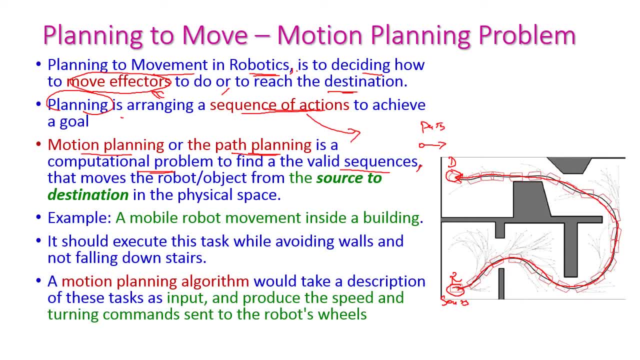 of actions. so what sequence of action the robot needs to perform to reach the destination right? and the movement is actually in physical space, that is, inside a building, for example. ok, for example, we can take automatic vacuum cleaner, so in the vacuum cleaner, how the vacuum cleaner will move inside the building, inside the building to clean the building. ok, so it. 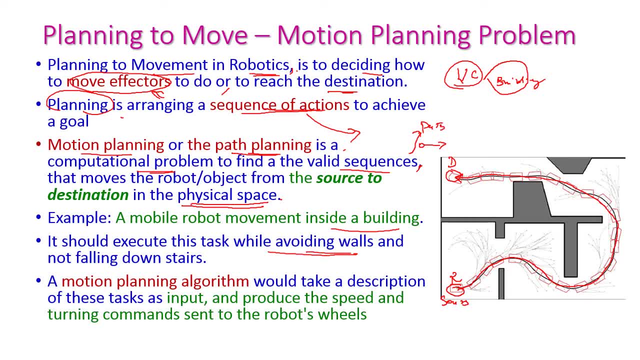 it should avoid walls and it should not fall down on the stairs. ok, sometimes steps may also be there. it should not fall down on the staircase or steps and it should avoid the walls. so these are the instructions we have to give as input. ok, so the motion planning algorithm would take descriptions of these tasks as input. so these instructions. 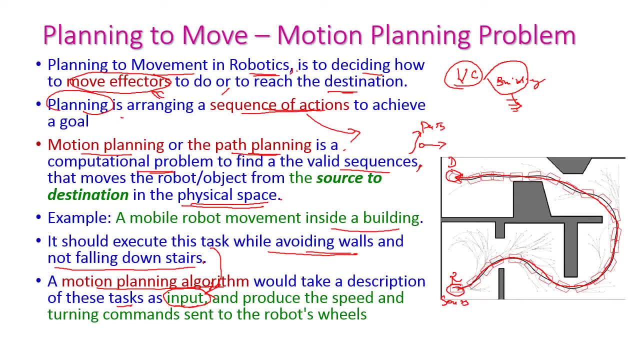 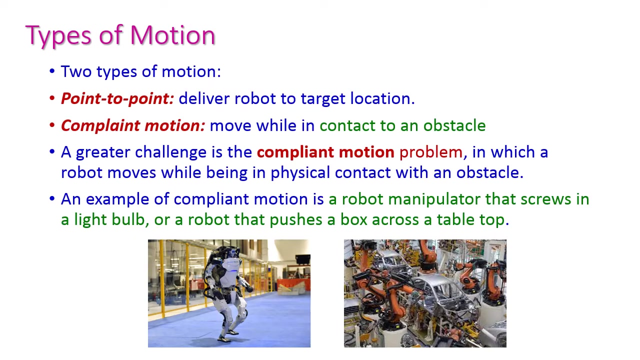 should give as input to the robot and it produce the speed and turning commands where to turn. ok, if it reach the wall then it should turn left side or right side, ok. so those turning commands and speed will be given to the robot wheels so that the robot can move from one place to another place inside the building right. there are two types of motions. the first one is point to point motion and second one is compliant motion. point to point means the robot can move from one place to another place inside the building right. there are two types of motions. the first one is point to point motion and second one is compliant motion. point to point means the robot can move from one place to another place inside the building right. there are two types of motions. the first one is point to point motion and second one is compliant motion. point to point means the robot can move from one place to another place inside the building right. there are two types of motions. the first one is point to point motion and second one is compliant motion. point to point means the robot can move from one place to another place inside the building right. there are two types of motions. the first one is point to point motion and second one is compliant motion. point to point means the. 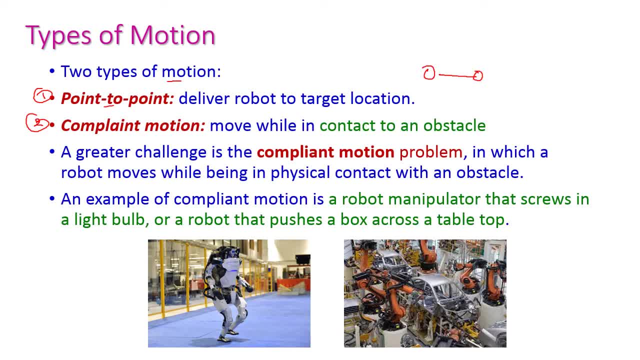 robot itself will move from one place to another place. ok, this is source, this is destination. so, if the robot itself will move from one place to another place is called as point to point motion. this is somewhat simple one, because the robot will move inside the building or outside the building, and second one is compliant motion. when come to compliant motion, the robot move while contact to an obstacle. ok, that is, the robot can carry an obstacle under the. 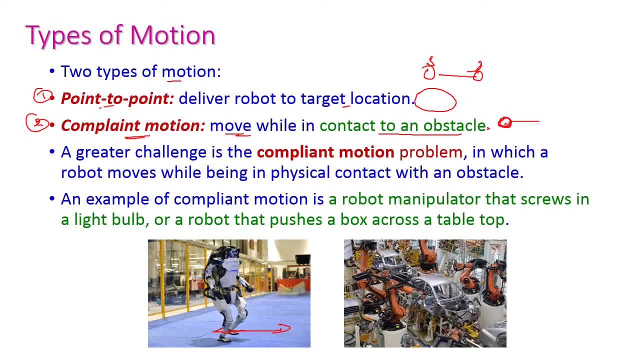 move, or the robot can do the obstacle while moving- okay, so this is somewhat difficult when compared to point-to-point motion. okay, and for example, the robot that screws the light bulb: okay, that is, the robot will fixing the light bulb. or the robot will pushes the box across the table, for example. you 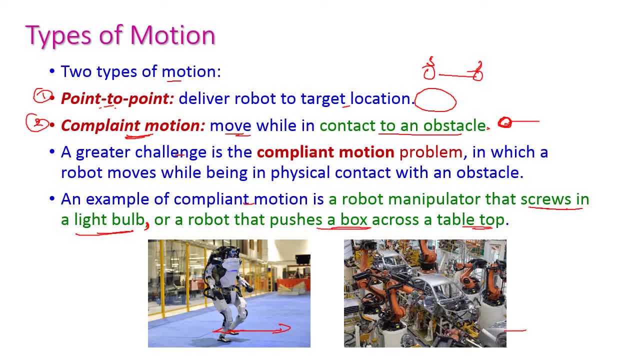 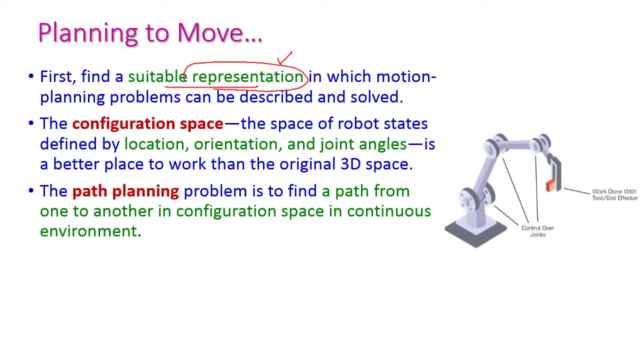 can see in this image, the robot is manufacturing the car. okay, by fixing all the screws, and the car will move from one place to another place. so all the robots will do some work because of this moment. all right, it is important to find the suitable representation of a robot, of a robot in which motion planning 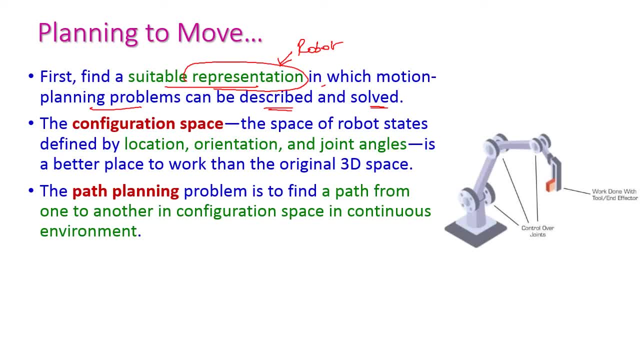 problem can be talked about a little more, or definitely otherwise. robots will can be described and solved. So ah, first we have to fix the configuration of robot, ok, and how it is represented, and those are decided in the beginning itself. So here two things are important. first one is configuration, space, second one is path planning. So configuration. 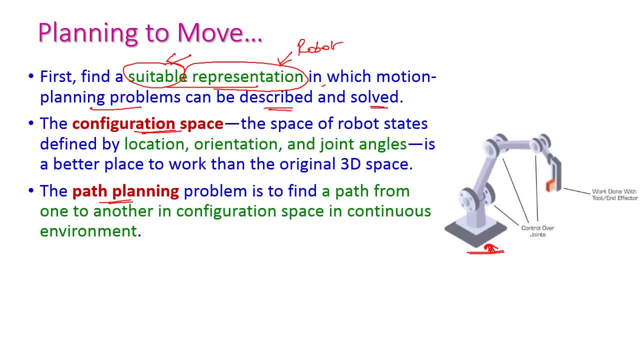 space means in which, ah how the robot is configured and in which place robot is going to fix Right. So the space of robot state defined by the location and the orientation, and joint angles. So based on the joint angle, only the robot can move right. So these things. 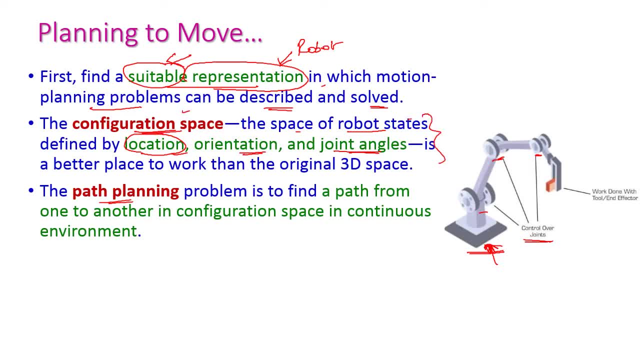 are very important, and this is called as configuration, space Configuration. space means the space where the robot is fixed, and next one is path planning. Path planning means the problem to find the path from So one to another. that is, initially, the robot is like this: after the ah, the movement, the 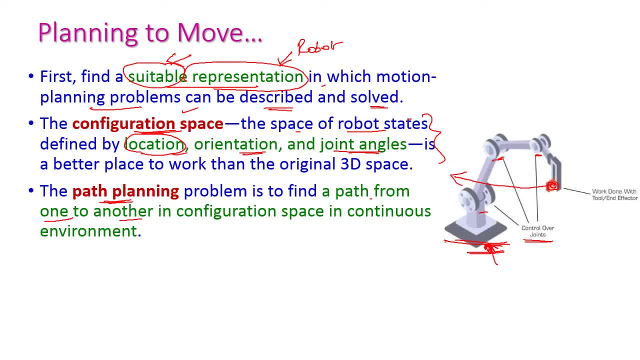 robot will move in this direction. in this direction, this is called as movement, and this is the path in which way the robot will move right, ah, in the configuration space. this is important in continuous environment. So here the environment is continuous. So configuration space means the space where the robot is fixed, and path planning means how the movement 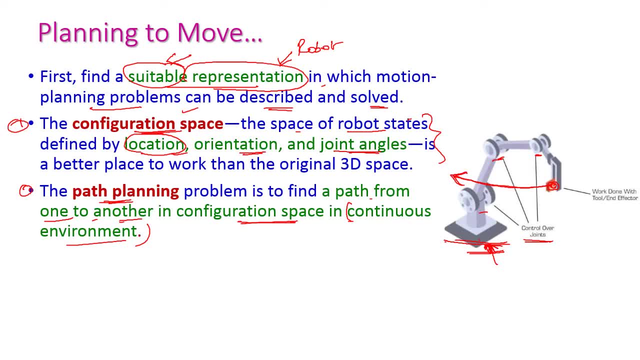 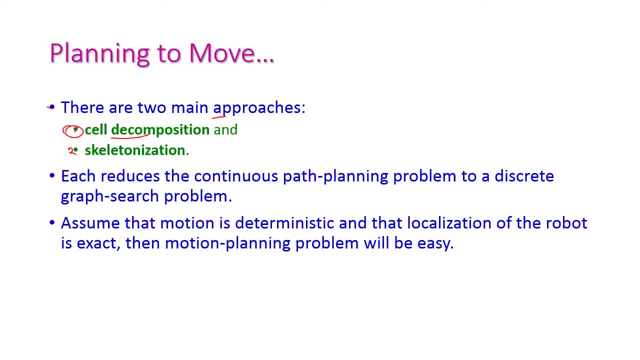 will be taken place. So these two things are important here. There are two main approaches in motion planning problem. first one is cell decomposition and second one is skeletonization. So these two approaches will reduce the continuous path planning to discrete graph search problem. ok, So if it is continuous path planning, 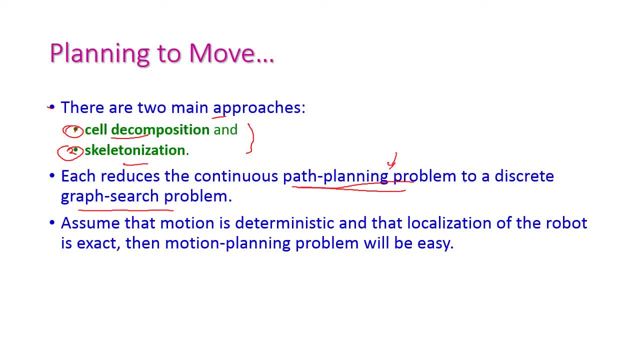 problem. this will be very much difficult, but if we reduce to discrete graph ah graph search problem, then the complexity will be very much reduced. ok, And it is also easy. if the motion is discriministic and the localization of robot is exact, ok, That is, if it is in exact location or exact fixed movement, then the motion will be very 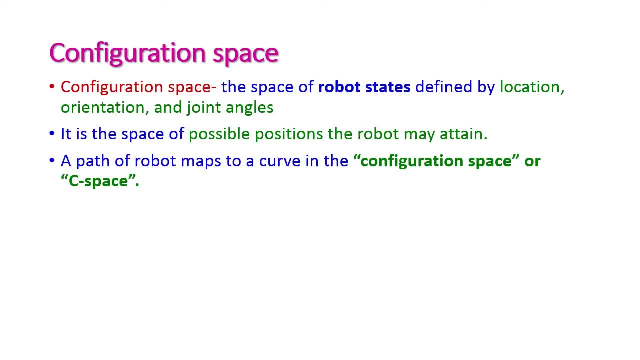 much easy Configuration space in robotic motion problem. the configuration space is very important and it is otherwise called as C space. right, ok, The configuration space means the space of robot states defined by. So the robot state should be defined by the location orientation. 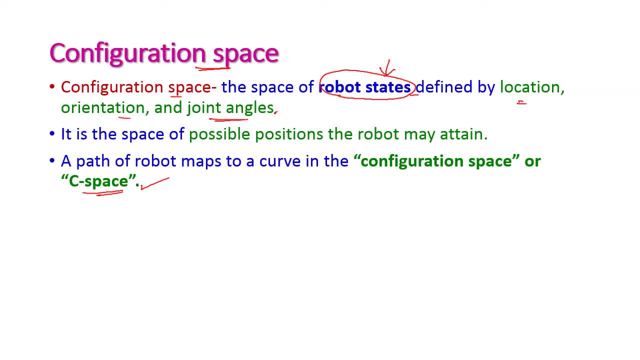 and joint angles. ok, So the space for defining all those things is called space. So we are is called as configuration space, right, And it is a space of possible positions. the robot may attack possible position. the robot may attack. right For explaining this configuration. 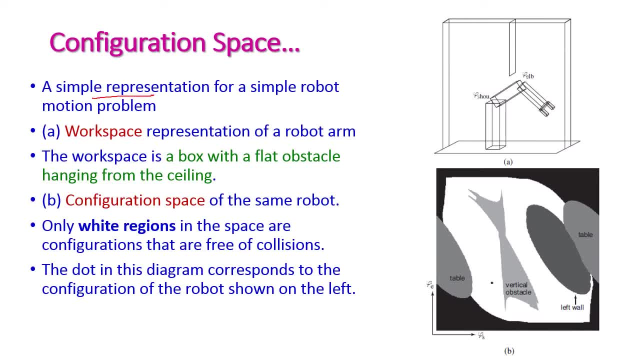 space. let us take one simple representation of a robot with a single arm, For example. this is our robot. the robot is having one arm. okay, robot with an arm. So this is our example And the workspace is this particular diagram. okay, workspace. representation of 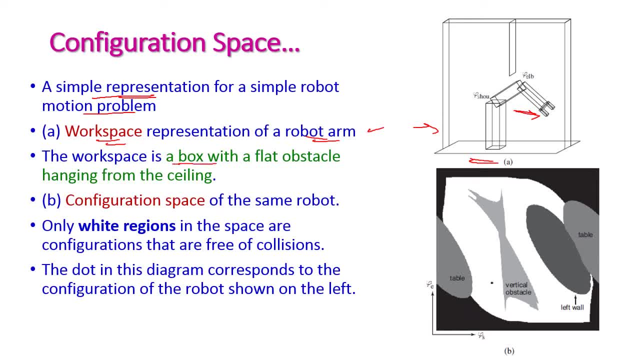 robot arm. The workspace is a box with flat obstacle hanging from the ceiling. okay, So this is the box. okay, In this box, the flat obstacle is hanging in the wall. okay, So this is what the workspace So. 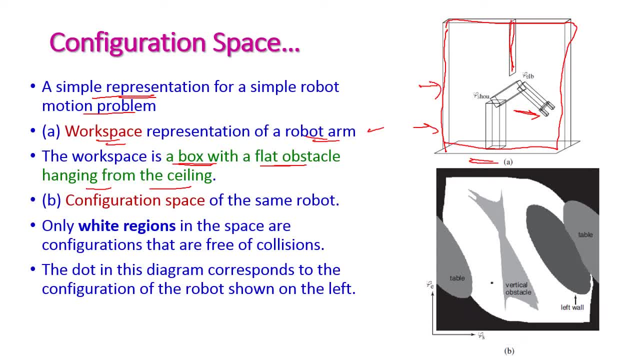 the robot is working in this space, in this box, where the robot is actually working is called as workspace. When come to configuration space, okay, So this is the diagram for explaining the configuration space for the same robot. right, The white region: see the white region. 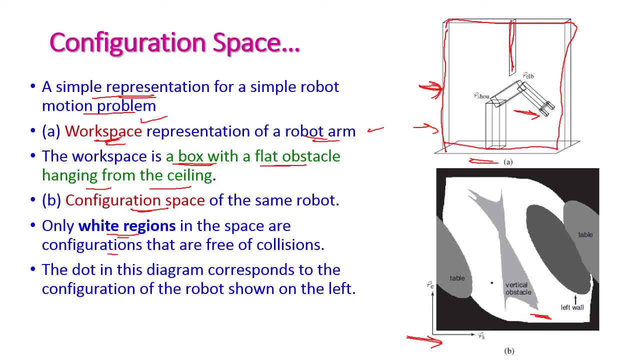 is the space for configuration that are free of collisions. okay, The white region free of collisions. there is no collision in this white region. right, The dot in the diagram- see the dot in the diagram. okay, corresponds to configuration of robot. okay, Actually. 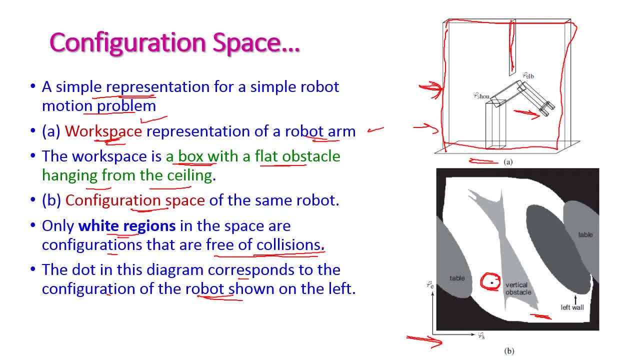 the robot is fixed in this space. okay, The robot is actually fixed on a table. These are the table and table. This is left wall. okay, the left side wall is this one, and vertical obstacle is hanging. that is here, okay, and the free space are represented as the white space right: The. 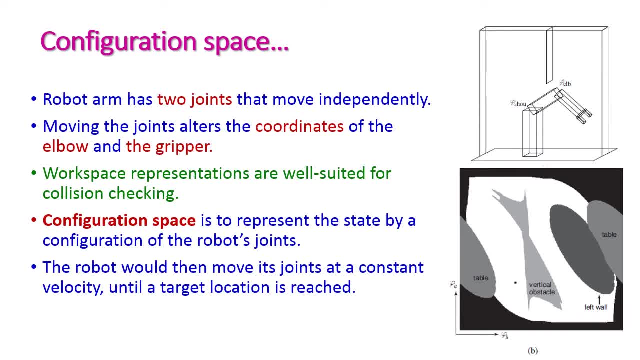 robot arm has two joints And that is move independently. for example, this is one joint and this is another joint right. So this is called as elbow joint sólo. to roll over, It is demonstrated as chiffon vertical combat zone, which will not be allowed because the 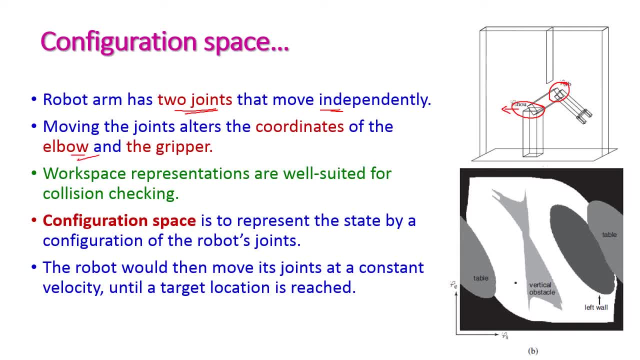 Austrian machine is made of aprove and SLение and the tray type, which is needle type, So elbow joint, and this is called as gripper joint. So when the arm moved from one direction to another direction, both the coordinates of two joints will get changed So that the 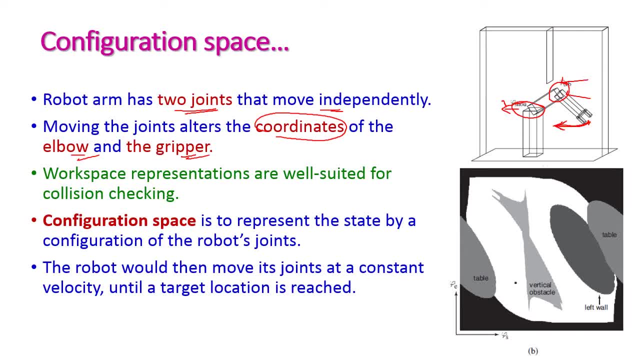 arm will move from one place to, that is, one direction to another direction. So this will be happen in workspace representation. that is workspace of robot. So the workspace representation are well suited for collision checking. And next one is configuration space. Here it 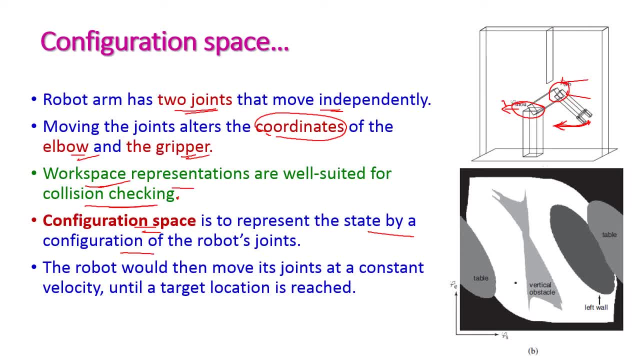 is represented the state by the configuration of robot joint. So the configuration space is used to represent the state of robot. How the state of robot will be computed By configuration of robot joint. How the robot is at present. What state The robot is at present, That is computed by using the configuration space, right? So 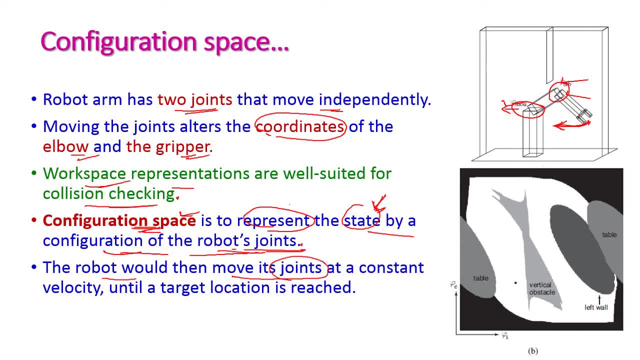 the robot would then move its joint and constant velocity. So for movement- suppose the hand will move from one place to another state- then it have to apply some constant velocity on that arm So that it will move from one location to another location until it reached. 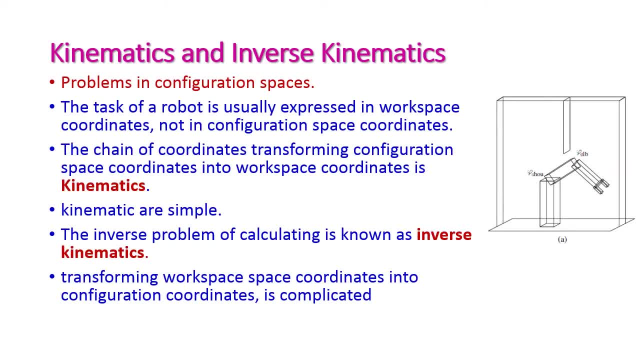 the target: The problems in configuration space. Normally the task of a robot is expressed in workspace coordinate, but not in the configuration space coordinate. ok, So it is important to transfer the coordinates of configuration space into workspace. ok, So that is configuration space. 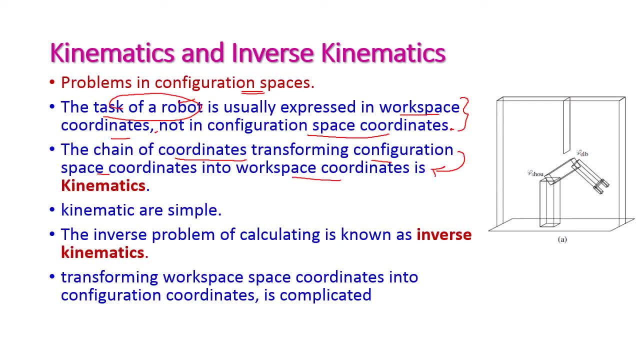 should be transferred into workspace coordinate. This process is called as kinematic. So kinematic is very simple one, ok. Kinematic means transforming the configuration space coordinate into workspace coordinate right. The inverse of this problem is called as inverse kinematic, Inverse kinematic. 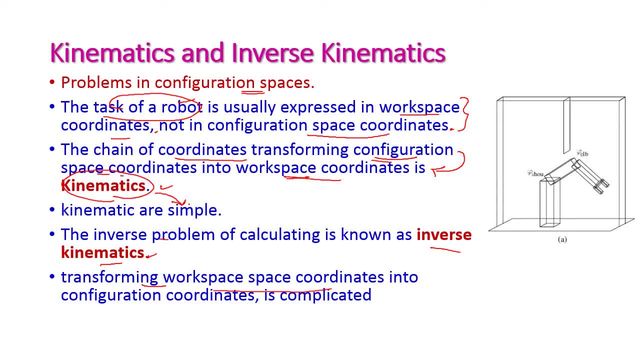 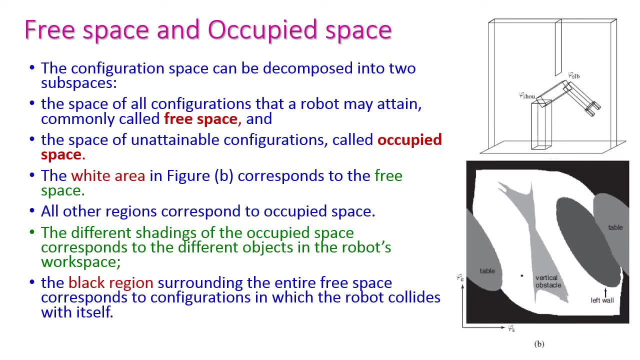 means transforming workspace coordinate into configuration space coordinate. but this inverse kinematic is somewhat complicated. one Thank you, And next let us see the free space and occupied space. See in the configuration space can be decomposed into two subspaces. First one is free space and second one is occupied space. 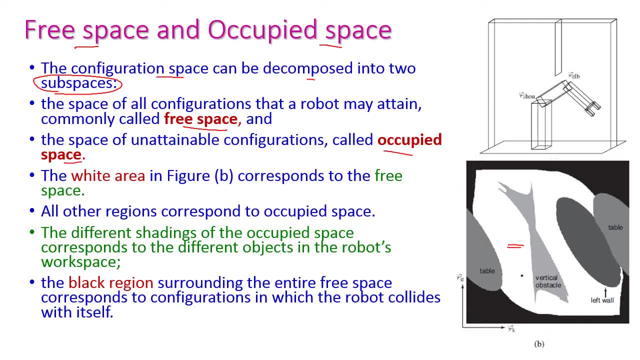 The white area are free space and all the shaded regions are occupied space. That is, the different shading of occupied space correspond to different objects in the robot workspace. So this region is occupied by table and this region is occupied by left wall and this region is occupied by right wall. 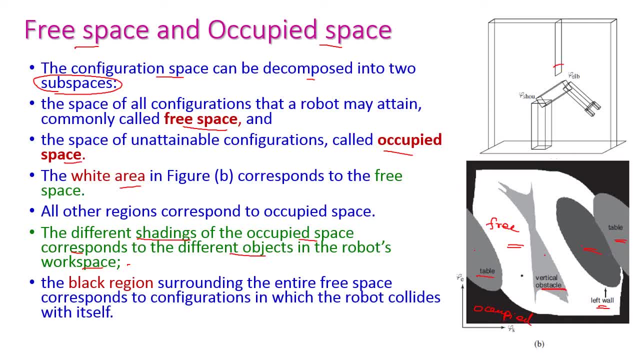 So this region is occupied by the vertical obstacle. This one, The vertical obstacle, occupied this region And the black region which is surrounding. See, the black region. These are the black region, Isn't it So? surrounding entire free space, which corresponds to configurations in which robot collide by itself. So if the arm extend in this level, then collision may occur. 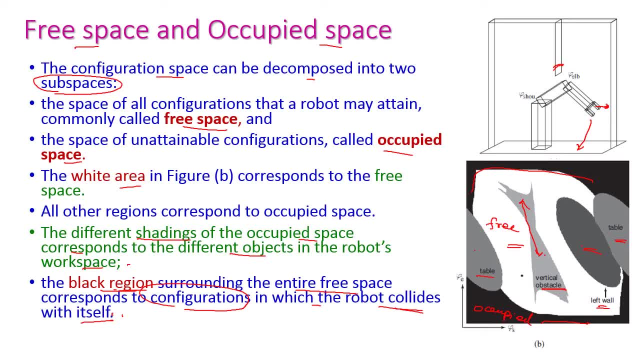 If the arm extend in this level, then collision may occur. That means it can touch the wall. It should not touch the wall While working or while taking some of the object. the robot arm should not touch the wall. Hence these regions are collision regions. 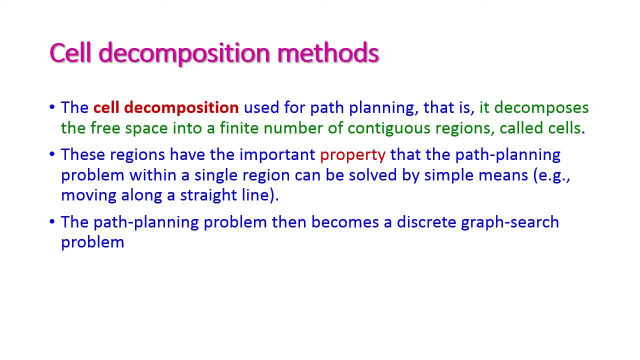 The next one is cell decomposition method. This cell decomposition is used for path placement. This cell decomposition is used for path placement. This cell decomposition is used for path placement. The next one is path planning problem. Path planning problem means the robot will move from source place to destination place. 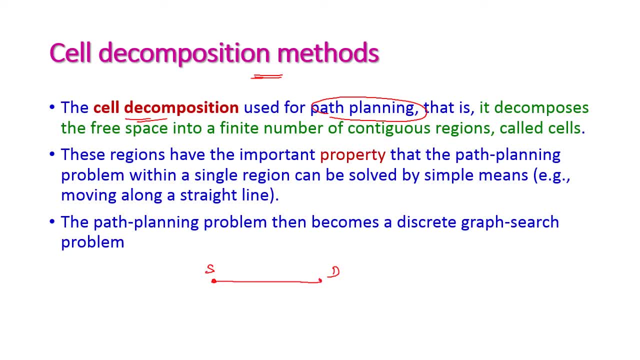 So it needs to identify the path from source to destination. Now the cell decomposition means this entire space will be divided into finite number of cells. Ok, By combining these cells, we can easily find the path from source to destination, So that the robot can use this path to move from one place to another place. 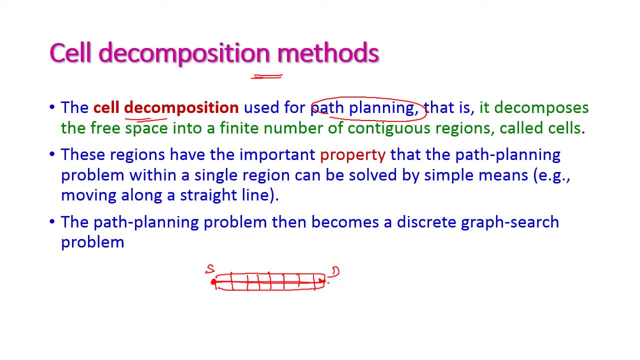 move from one direction, sorry, one place- to another place, right, and this one is called a cell, and these regions have some important property that the path planning problem with single region. so with the single region it is having some important property to solve by simple means. by combining all the means, we can get the path from source to destination. 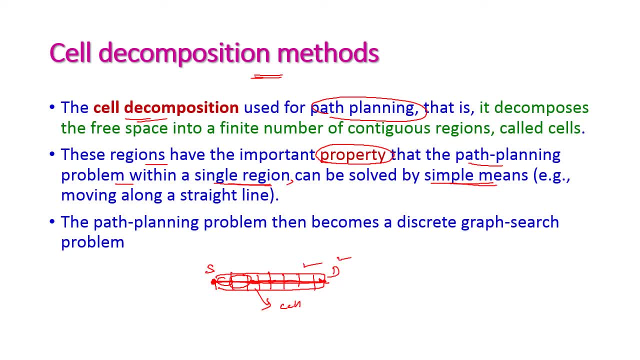 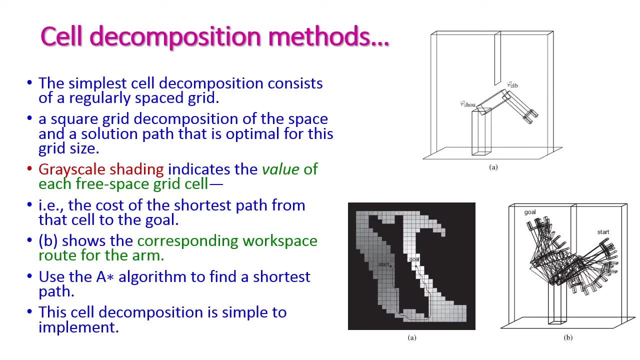 okay. and this path planning problem then become discrete graph search problem. so in the graph we can easily search source to destination, that is, path from source to destination, right? so the simplest cell decomposition consists of regularly spaced grid. see, the grids are constructed like this. okay, in this diagram each square is represented as a. 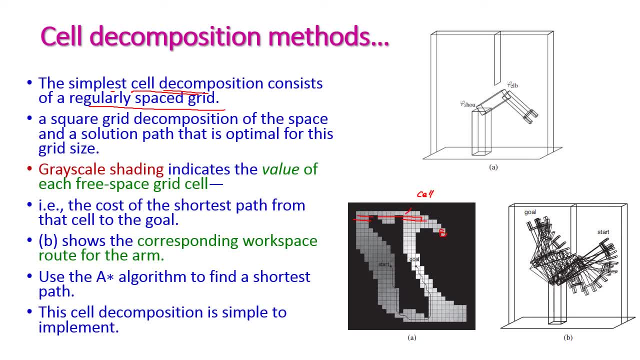 single cell. okay, the cells are arranged in grid form, right, and the squared grid decomposition of space and a solution path is optimal for this grid size. okay, so here, this is the starting place, and from the starting place the, the, the robot arm, have to move like this: okay, and finally it will reach the goal place. that is the. 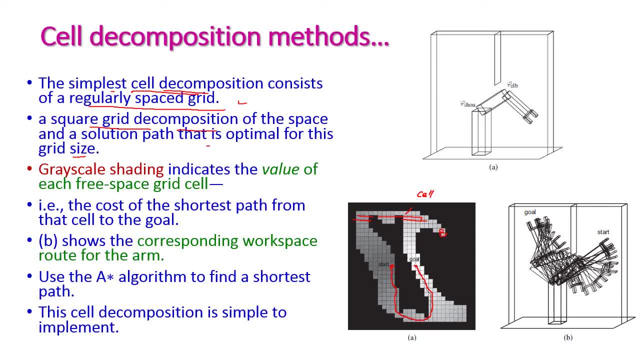 destination, because this grid will be arranged only in the free space. free space or white space. okay, so, because in the free space only the robot can move and it is important to find the cost of shortest path from start to goal. right, and this particular one diagram shows the corresponding workspace route of the arm. so the starting space to the arm will be moved in this way. okay, so, likewise it will reach the destination place. so for this, 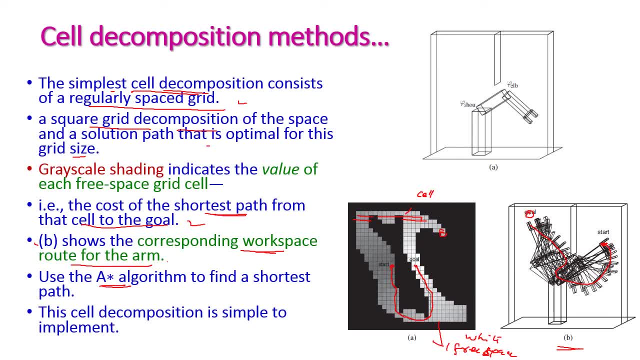 finding path from source to destination. we can use a star algorithm, right? So what is the purpose of a star algorithm? It is used to find the shortest path from source to destination. okay, This cell decomposition is simple to implement. And next let us see the limitations of cell decomposition methods. There are three. 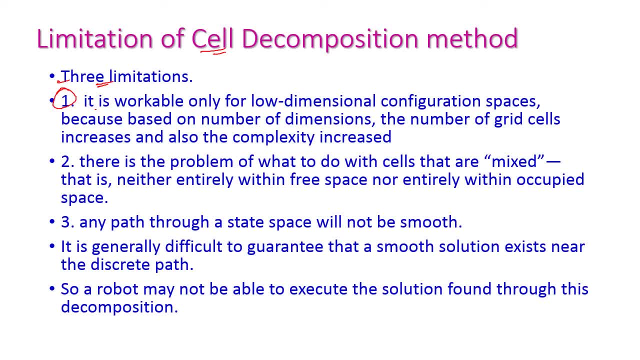 important limitations here. The first one is this: cell decomposition is workable only for low dimensional configuration. That is, if the configuration is two dimension, then it is easy to implement. Suppose, if the dimensions are increased, then the number of grid sets. 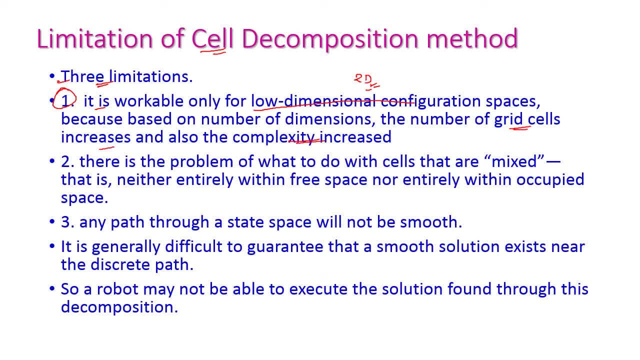 will also be increased, Hence the complexity will be increased. So it is workable only for low dimensional configuration space. And second one suppose if we implement, that is if the space is divided into number of cells, the cells will be more complex. So 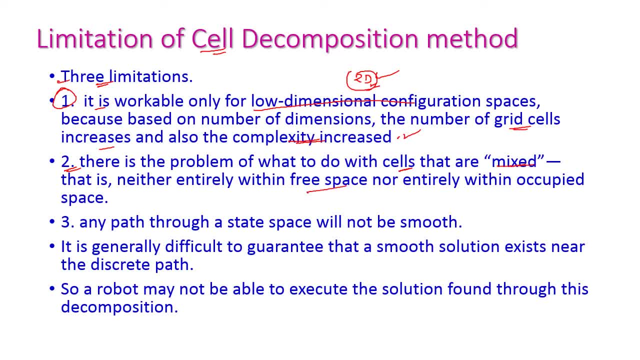 the number of cells will be more complex. So the number of cells will be more complex. So this concentration must be mixed in white space and the occupied space. Then it is very much difficult to count this particular cell for our configuration or for path finding. 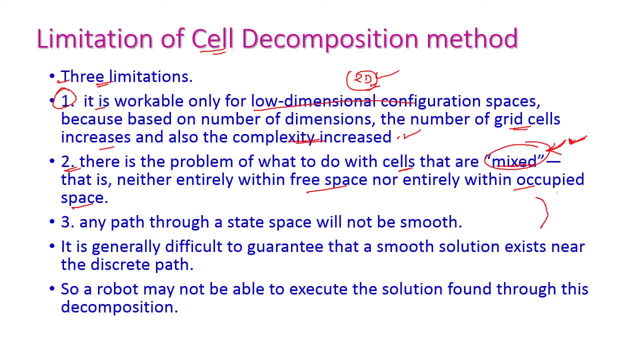 okay, For example, this is the free space. Suppose the grid is like this, So we cannot use this particular grid for five propor type. the path right, collision may occur. and third one: any path through state phase will not be smooth. okay, so the starting space may be here and destination may be. 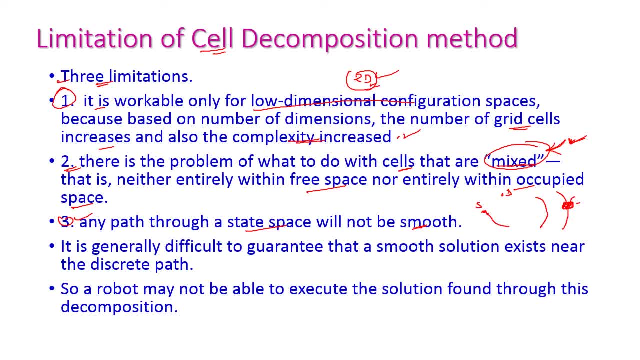 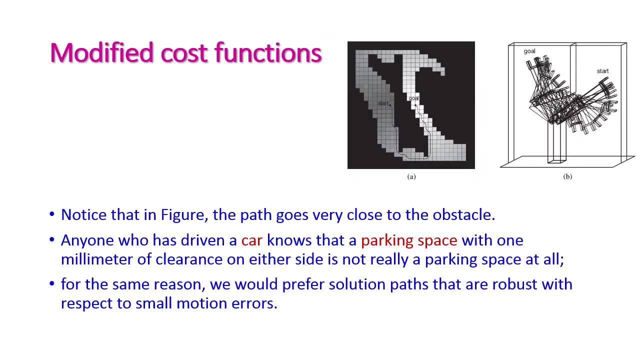 here. okay, the path may be like this. the path may be like this: not the straight line, right. so these are three very big limitations of cell decomposition methods. the next one is modified cost function. so to overcome the problem of cell decomposition method, we can move to modified cost function. okay, let us see. 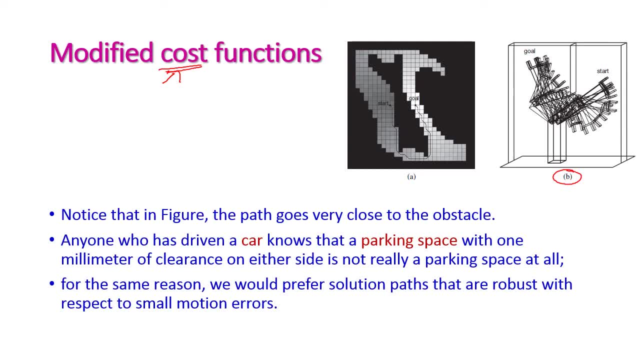 this particular figure here, the path from start to goal. see this particular path. this is very much close to the obstacle. see, these regions are very much close to the obstacle, right, for example, this is the parking area of your car, this is parking area. in this parking area, this is exactly the size of the car. 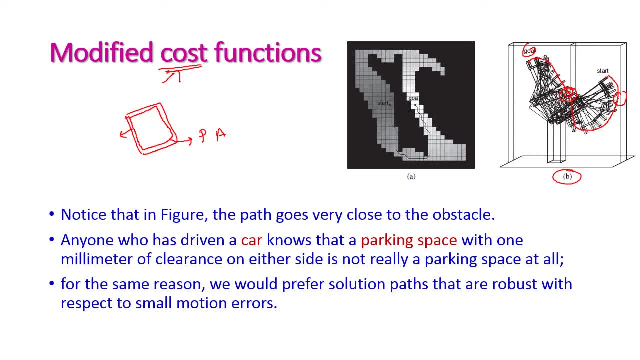 ok, only one millimeter gap, both safe. if the size, that is, the gap, is only one millimeter, then we cannot consider this parking area is a for this car, isn't it see? for the same reason we would prefer solution path that are robust with respect to small motion error. see if the error is very. 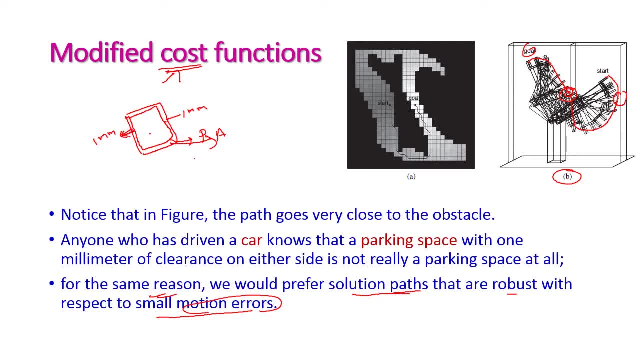 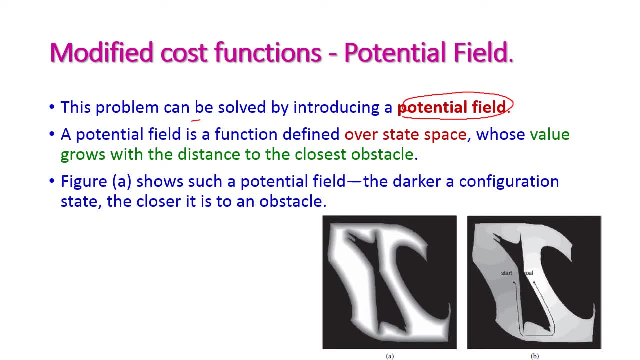 small, then the entire system will get collapsed. this problem can be solved by introducing potential field. potential field means see, for example, the white region is called as free space. so in the free space we are going to find the path from starting to goal state. so this is the starting and this is the path, okay. 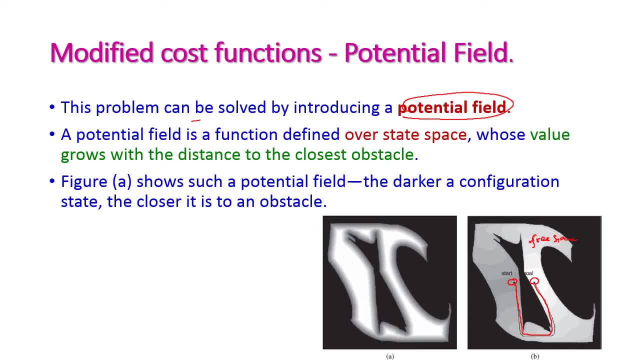 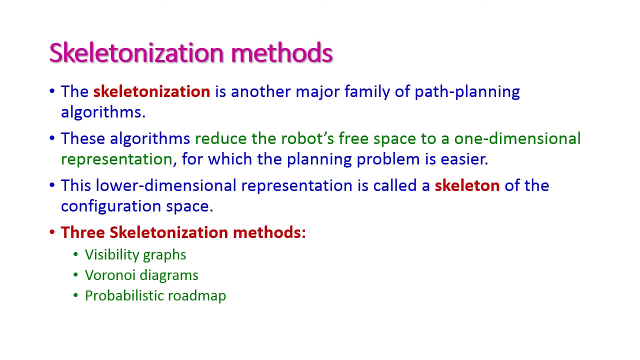 so here we introduce the potential field. so this is the shading. gray shading is called as potential field, potential field and in the potential field the value grows with the distance to the closest obstacle. so if it is closest to here, then the value will get increased. skeletonization methods. skeletonization is another important family of path. 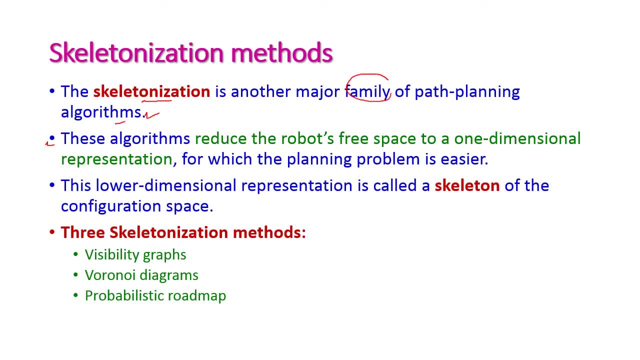 planning algorithms, and here this algorithm reduces the robot free space to one-dimensional representation. see, if it is one dimensional representation, the path planning is very easier, isn't it? so in the single dimension, we can easily plan the path of a particular robot, and this lower dimensional representation is called as. 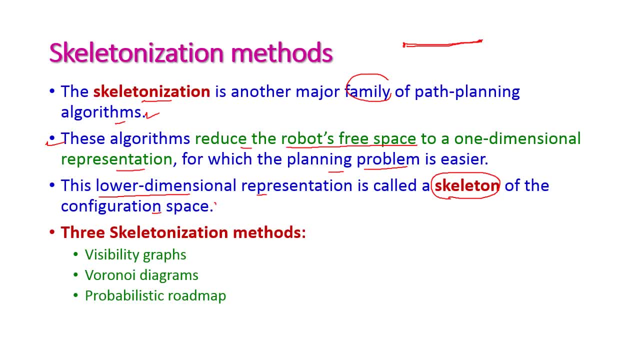 skeleton, skeleton of configuration space right. so the higher dimension will be reduced into lower dimensional space, so that finding path will be very easy. skeletonization methods: there are three different methods here. first one is a, one is visibility graph. second one is voronoi diagrams and third one is probabilistic roadmap. 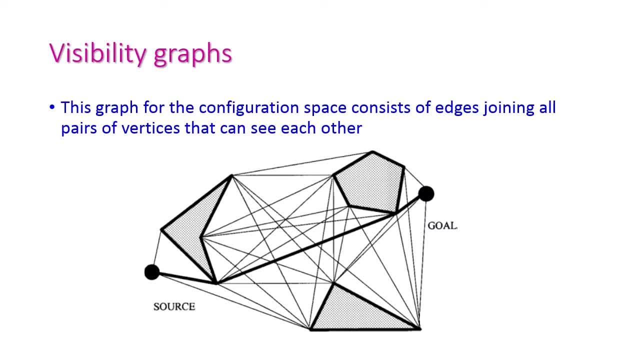 let us see all those things one by one. visibility graph: this is the first method of skeletonization here. this graph is for configuration space, so this is for configuration phase, which consists of edges. these edges will join all paths of vertices. okay, see, these are the vertices, and vertices are. 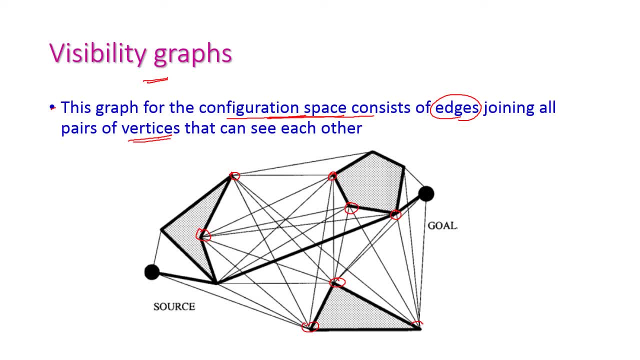 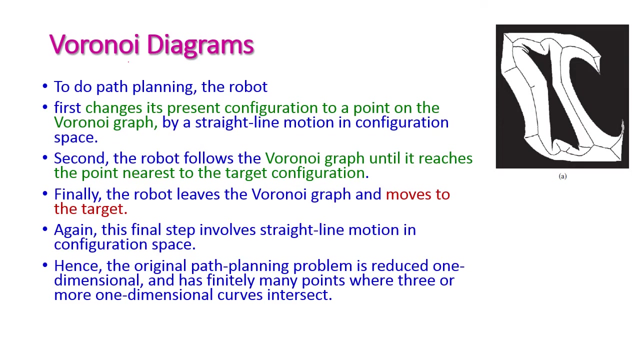 connected with the edges, more number of edges so that we can easily identify more path from source to destination. okay, so the path is clearly visible. see, this is another path. okay, directly we can reach the goal. so this is called as visibility graph. the second method, of skeletonization, is where an eyebrow here to do path planning. 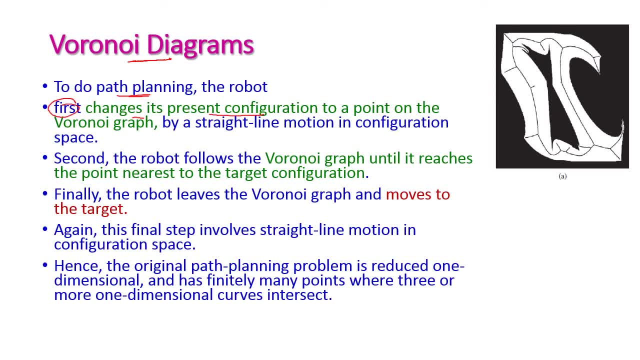 the robot first changes its present configuration into point on the veronigraf. okay, so first it will identify the points by using veronigraf, by straight line motion in configuration space. so the point should be joined by by using straight line, ok. and second the robot follows the vernon graph until it reach the 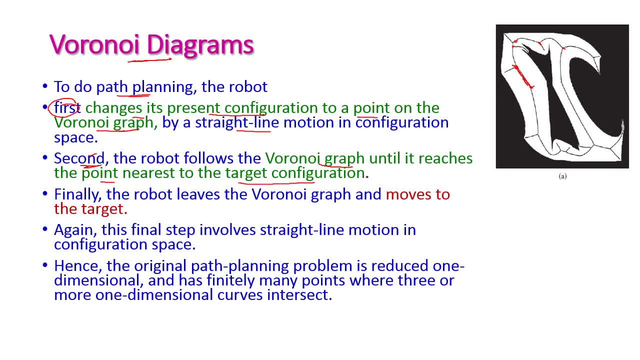 point nearest to the target configuration. see, for example: this is source and this is the target. ok, so from the source it will identify the nearest point to the target configuration. from here it will identify nearest point, ok. likewise, it finds the straight line motion in the configuration space to reach the target. that is the destination. hence the original. 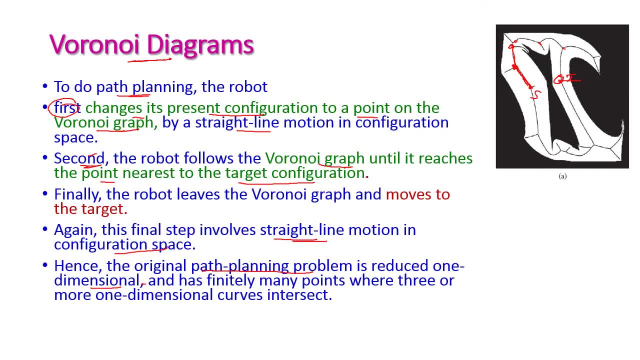 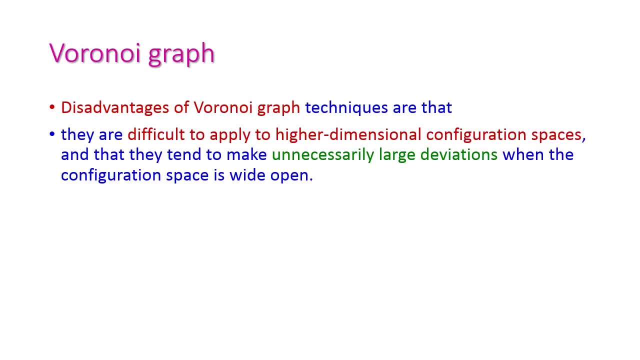 path planning problem will be reduced to one dimensional, hence more number of ah. one dimension curves will be intersect to each other to find the path. see the disadvantage of vernon graph and when come to large dimensional configuration space, it is very difficult to implement. ok, ah, because 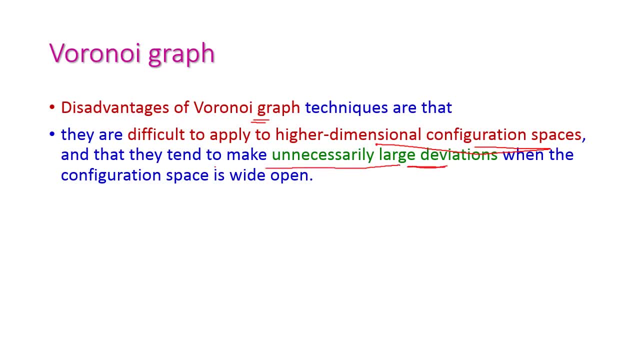 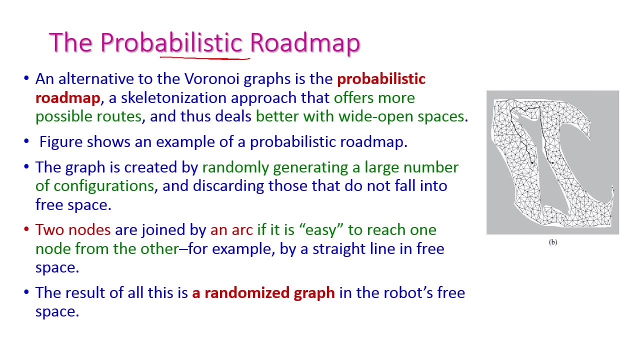 ah, they make unnecessarily large deviations when the configuration space is wide open- ok, so this is very difficult if the configuration space is higher dimensional. the third method of skeletonization is probabilistic road map. this is alternative to vernon graph. ok, this offers more possible routes and it can deal better with wide open spaces. so this is the alternative to vernon graph.